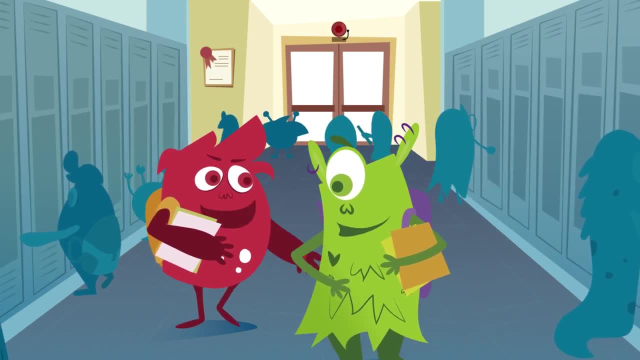 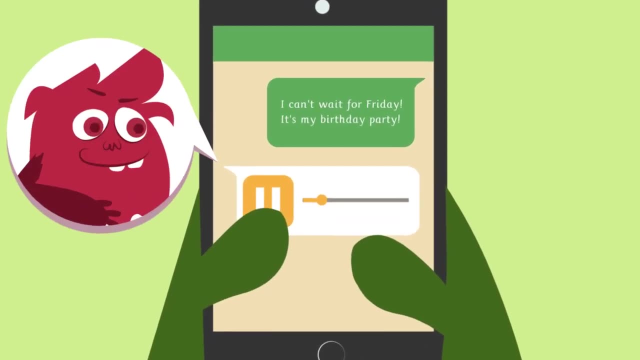 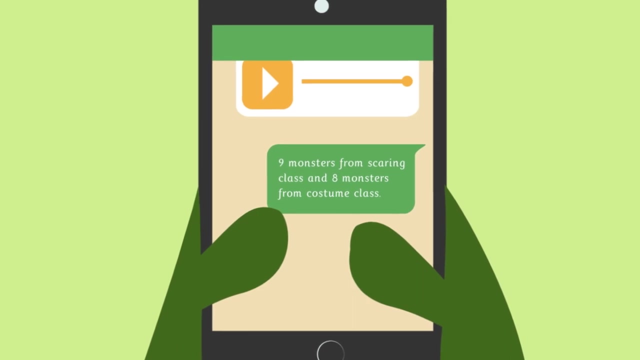 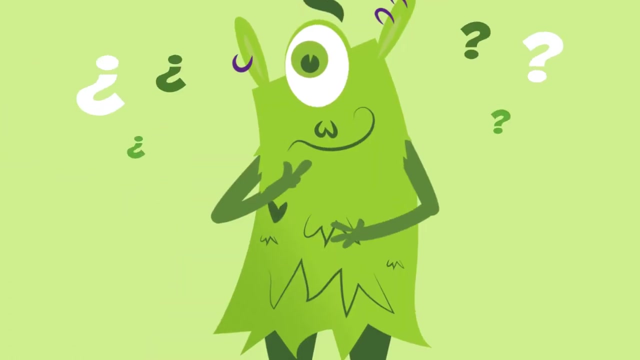 Oh, I have scaring class. I don't want to be late. We will talk later. So how many monsters are going to the party? How many invitations do you have to send? How many monsters do I need to send party invitations to if I want to invite nine classmates from scaring class and eight classmates from costume class? 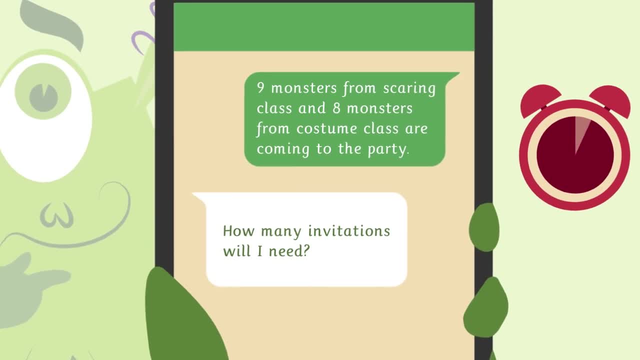 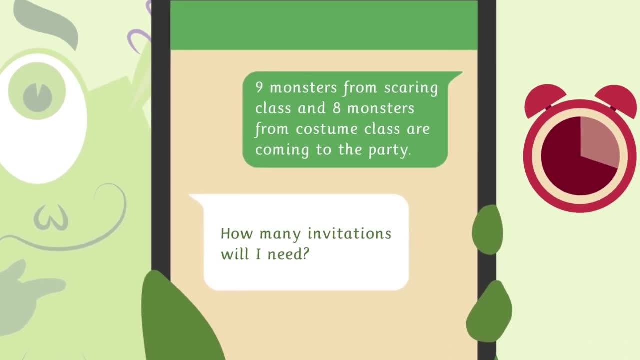 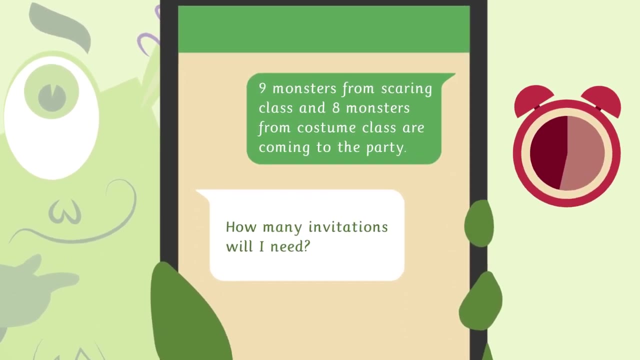 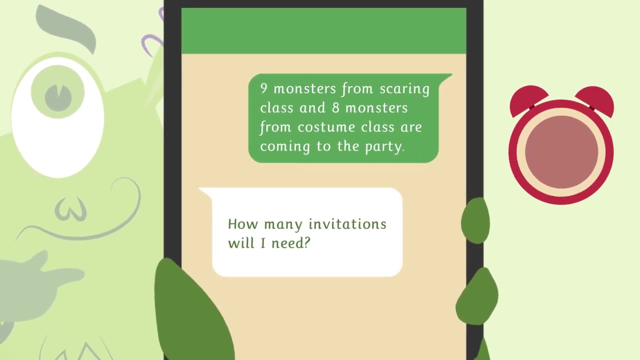 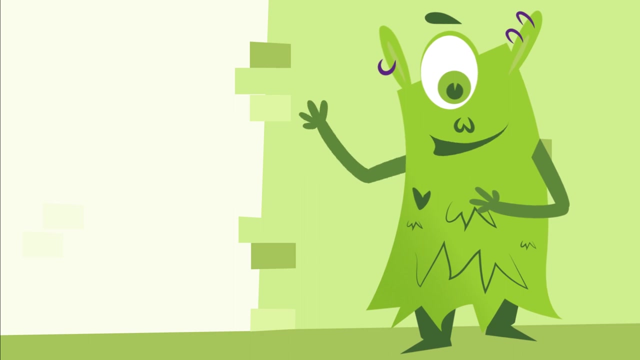 I'm worried about that. Excuse me, Wh comme Carry, Hurry up to your roaring customers. Oh, what's up todos? Hey Onil From Awara Sports Club. I am Chiara Cette, A professor. To know how many invitations I need, I have to add up the number of monsters I want to invite. 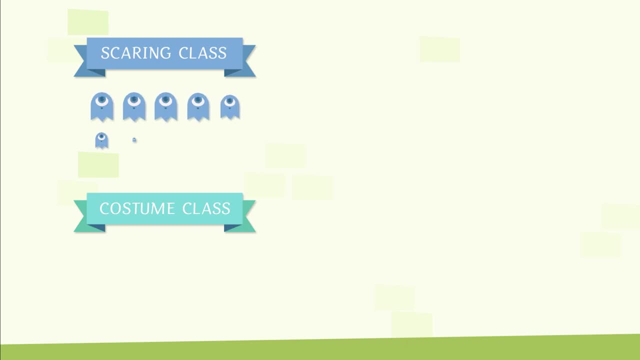 From scaring class, I am going to invite 9 people And from costumes class, I am going to invite 8 people. Let's add, We're going to add If we have 9 monsters in the scaring class and 8 monsters in the costumes class. 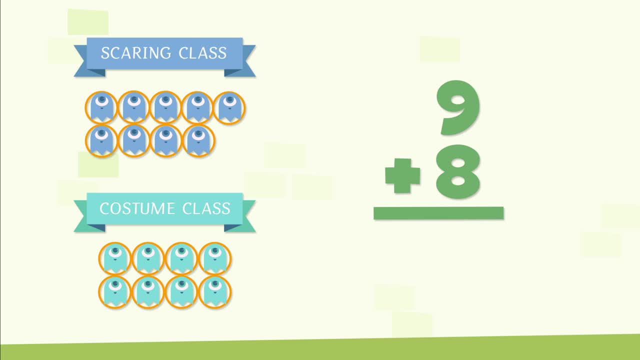 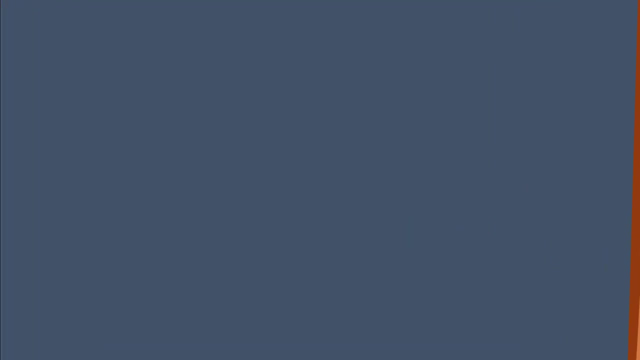 9 plus 8 is 17.. Let's put 7 here in the units column and the 1 in the tens column. Great, There are 17!. So 17 monsters are coming. Ellie and Little Blue told me they can't come. 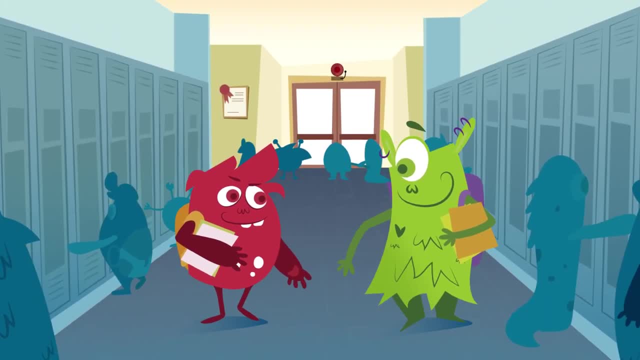 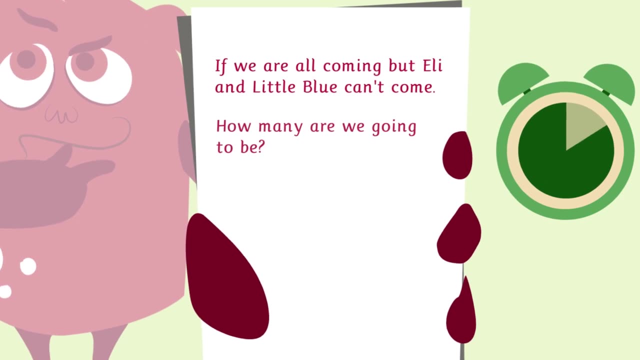 So how many are going? 7 monsters are coming. 積을때 4개의, 이은때 6개의, 이은땐은 7 개의, 이은땐이 12개의, 이은땐이 4개가 됩니까. 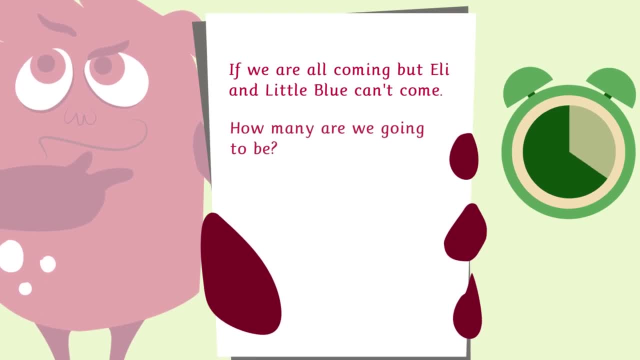 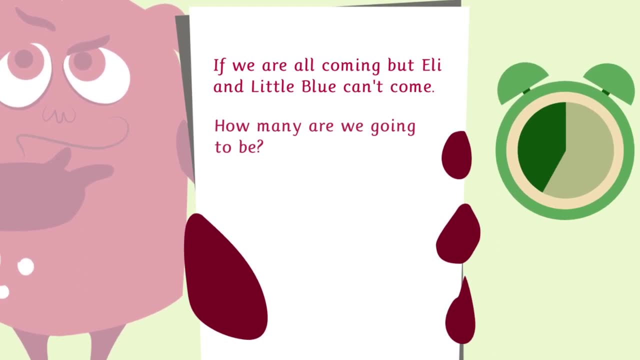 Например, 이는 이은땐, 어린이의 이은땐을 1명으로 이루는 것입니다. Let's add 6 monsters, 8 monsters, 3 monsters, 1 monster, 1 monster, 2 monsters, 3 monsters. 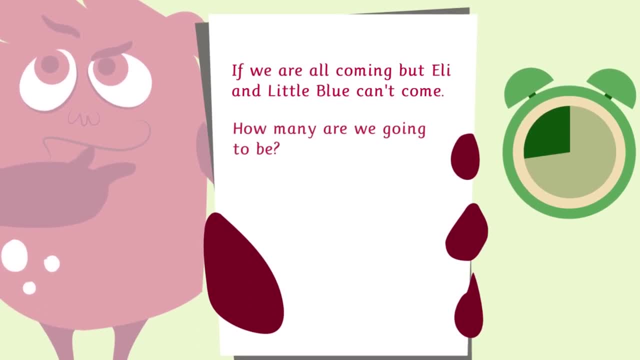 Let's add 6 monsters. 2 monsters, 2 monsters. 1 monster, 2 monsters. 3 monsters- 1 monster, 1 monster, 2 monsters. Let's add 6 monsters to the group, so we can add one more monster.